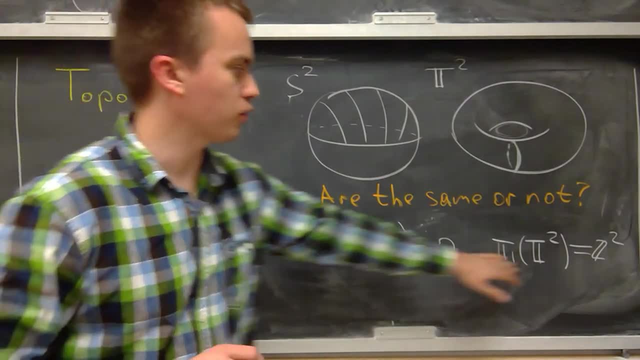 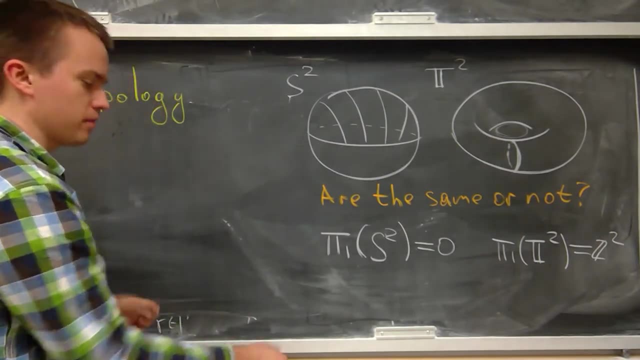 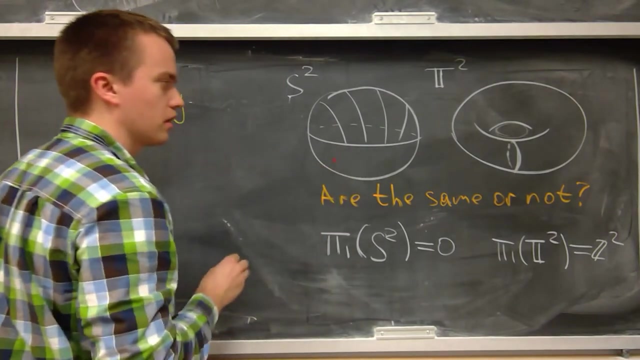 And we can see, since fundamental groups are different, that means that these two surfaces are different, And let me just show you one more example. Let me just tell you what the fundamental group is. So fundamental group is basically saying that let's take some any point in my space, in other. 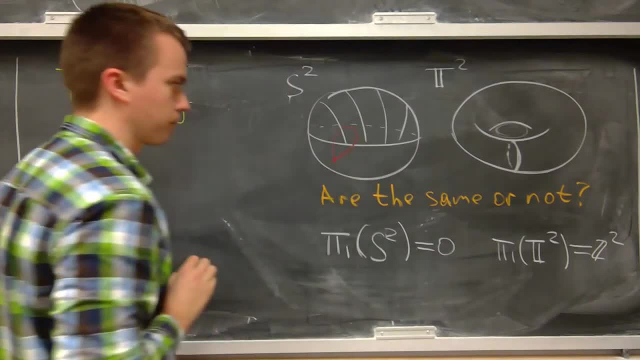 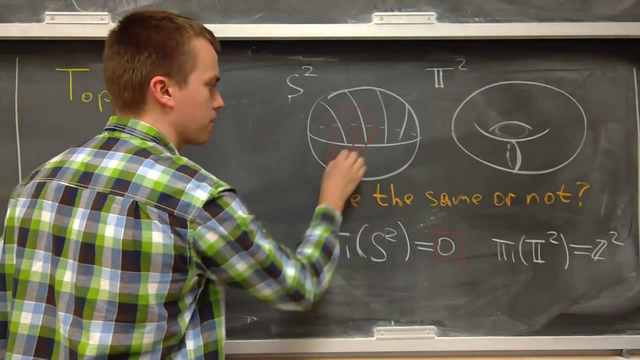 forms of my surface and I will draw a loop Then. fundamental group of S2 is trivial because you can see, for any loop that you take, you always can shrink this loop to a point. So you take a loop and you shrink and you get a point. 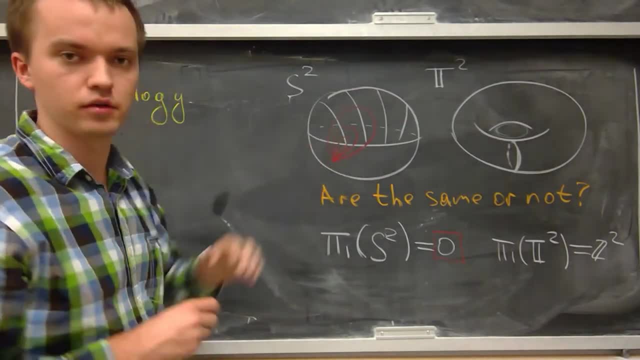 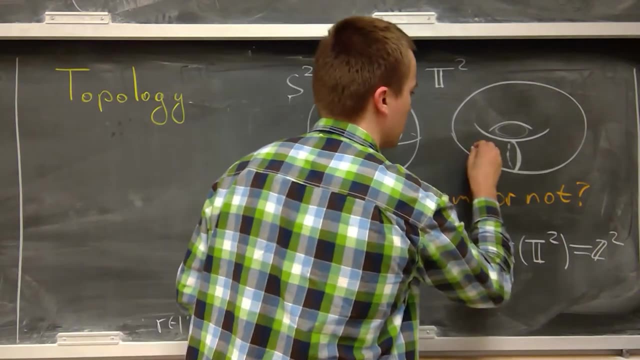 And this is true for any point in the sphere, And this is true for any point in the sphere And for any loop. But here on a torus, you can see so that if I will take, for example, like this loop, Then I can't shrink this loop to adapt to a point. 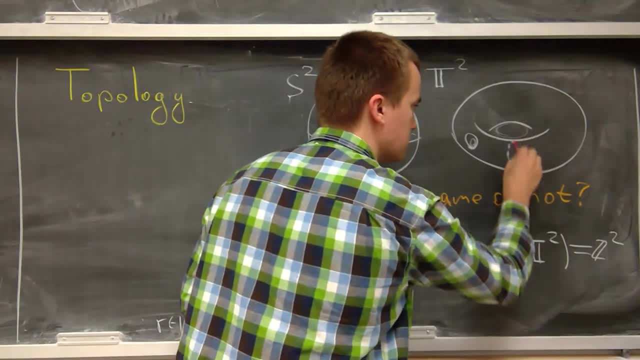 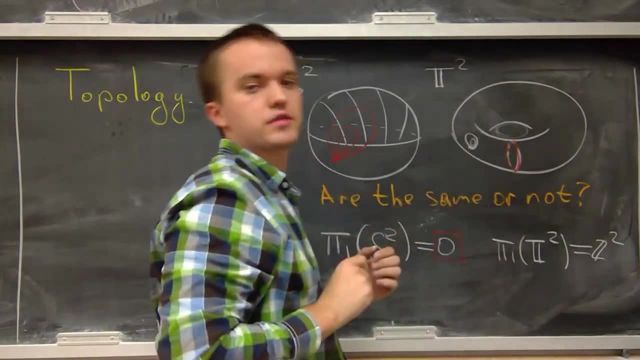 But if I'm going to take this loop, it doesn't matter how I'm going to move this loop around the torus. I will never be able to shrink this point to adapt And you also can see that I have 2 loops of such kind. 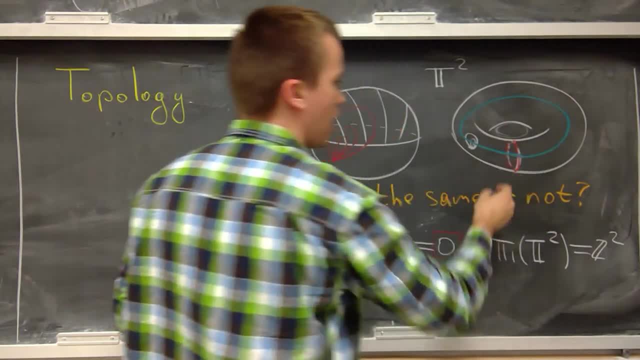 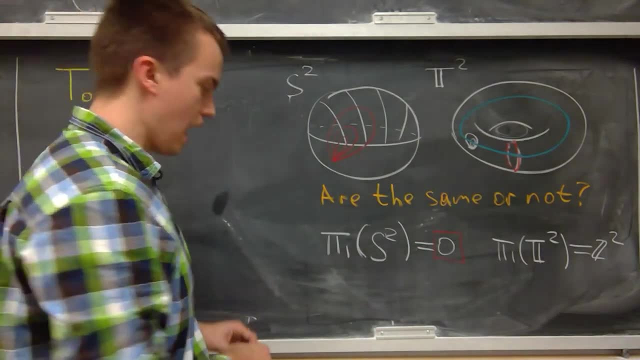 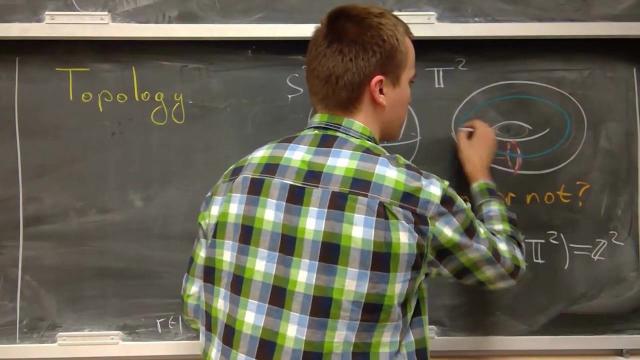 I have this loop, Or I have loop 2 loops, that goes around this empty space, around the circle, And that's why I have Z two, because one Z generated by this loop and another G generated by this loop. So this type of surface are really difficult. 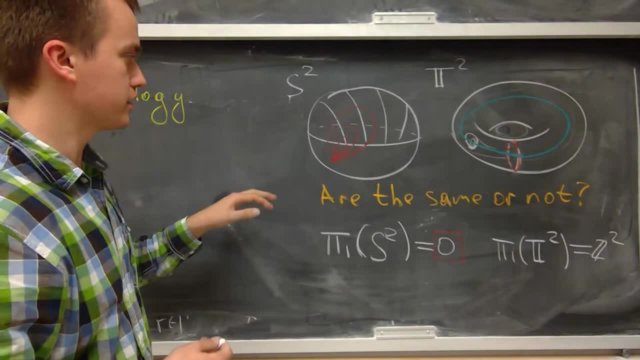 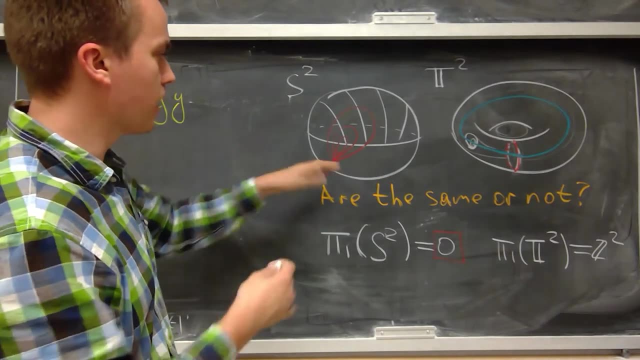 And let me show what path leads us to be able to use this tools. and what do we need to study in topology if you want to be able to apply these tools and to be able to distinguish like two surfaces, like two manifolds, topological spaces? 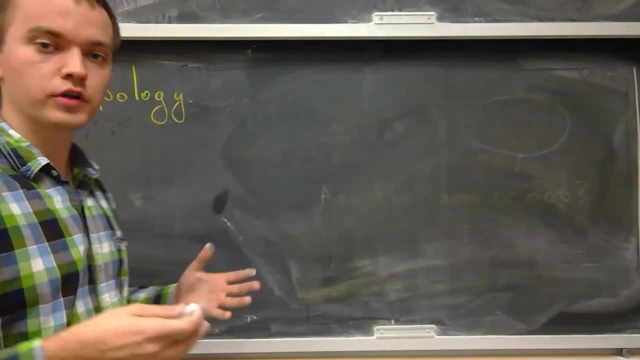 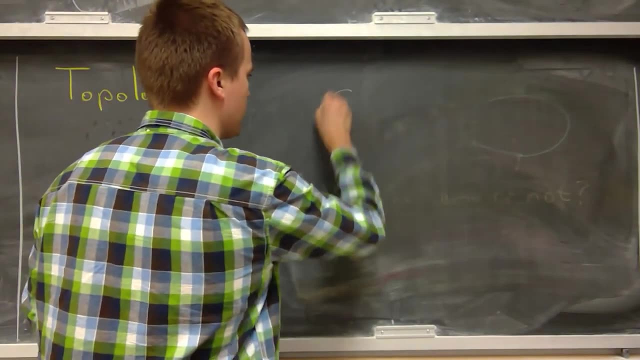 that they're the same or not. So in order to show this, how to distinguish like big ones, let's first draw small ones. Let's first, let's say, draw a circle which is like just S one and a line interval. 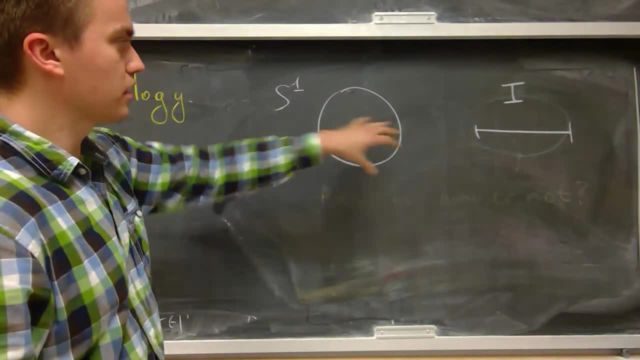 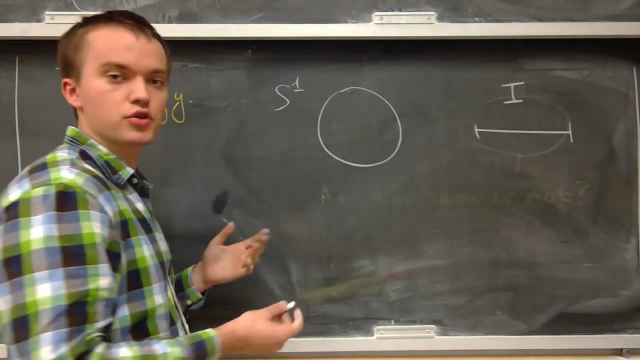 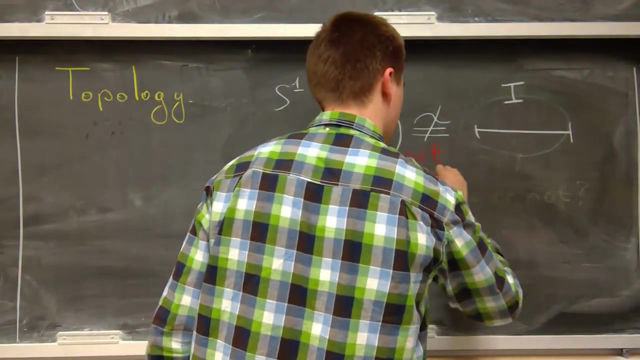 And what I want to say about this. I want to say that this two, like spaces, like this is, two objects are not the same. So I want to show that there are not homeomorphic. And what does it mean homeomorphic? It means like there's exist a mapping between two spaces. 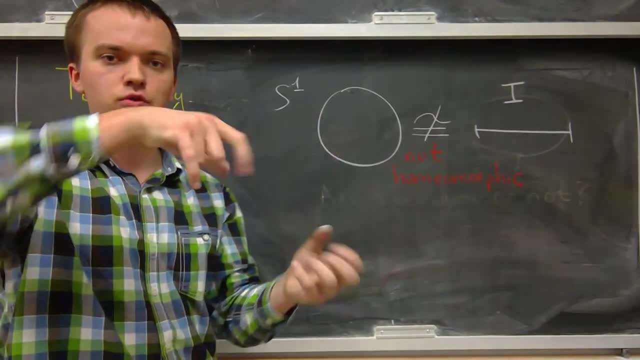 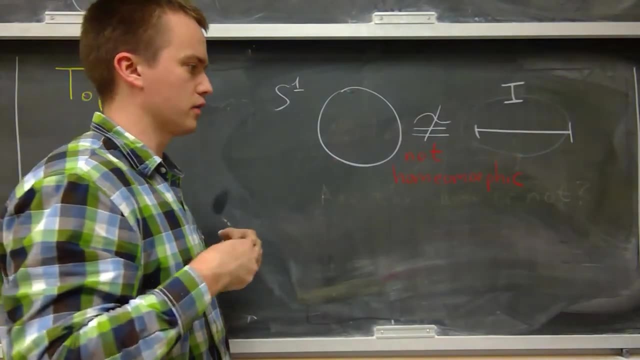 And this mapping. you can think about it. You can take one space and you want to deform it. You're not allowed to break it, You're not allowed to cut it and reattach. So the only like transformations that you can do. 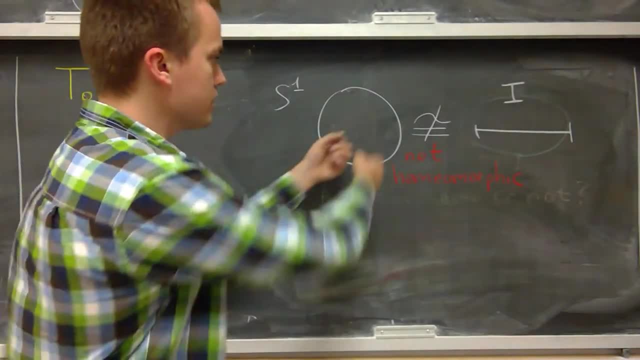 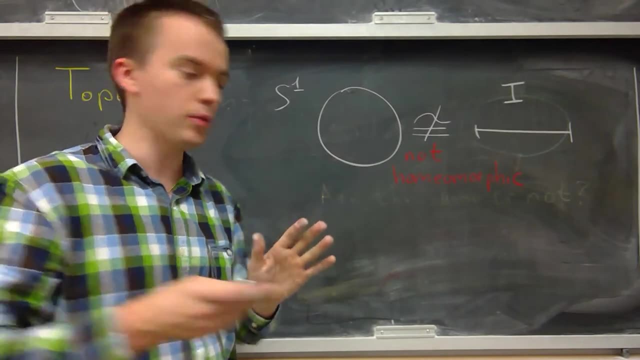 you can squeeze it, You can make it smaller, bigger and you can see if I will take the circle and we'll try to rotate. I will never make the circle to be aligned, But you will ask: there is one way Because I can have. 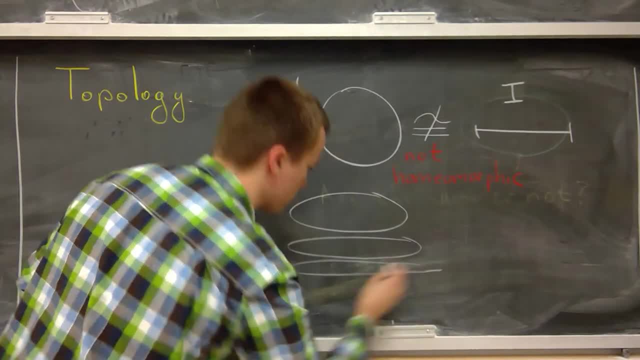 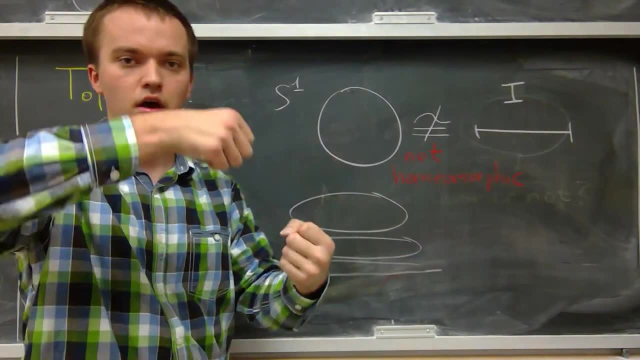 I can take my circle and just make it smaller, smaller and smaller, So kind of map my circle into unity interval. Yes, but being homeomorphic means every time you do this transformation, your transformation is bijective. So you can have multiple systems. 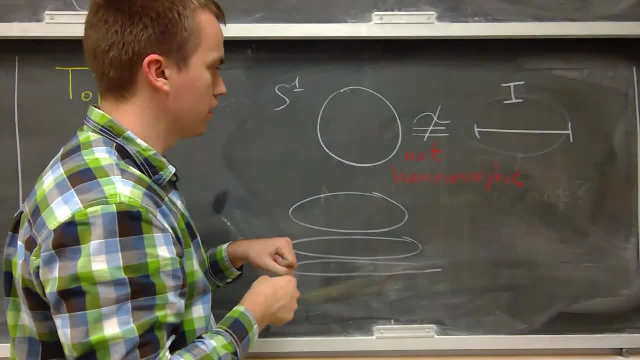 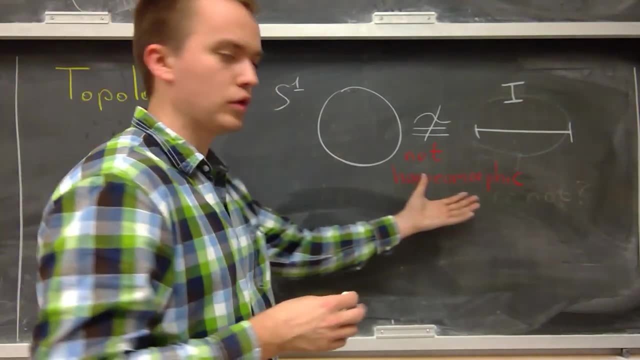 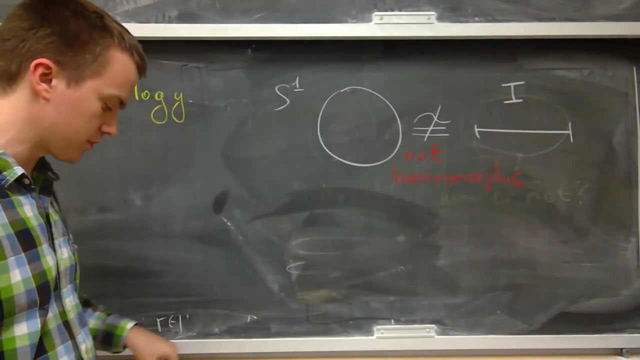 so you you never overlap your points and if you understand what this objective means, then, like this, map must be bijective. so we want to study some maps and these maps required some space. so topology is the first thing that we study. in topology we study topological. 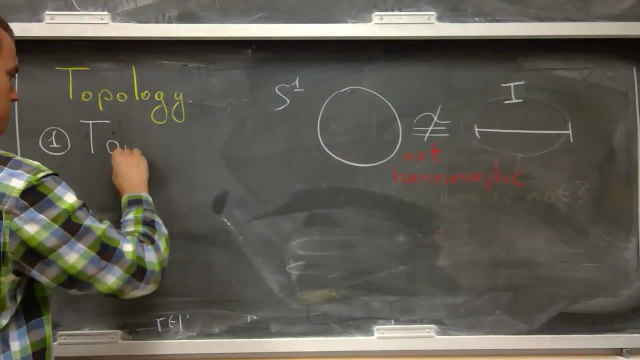 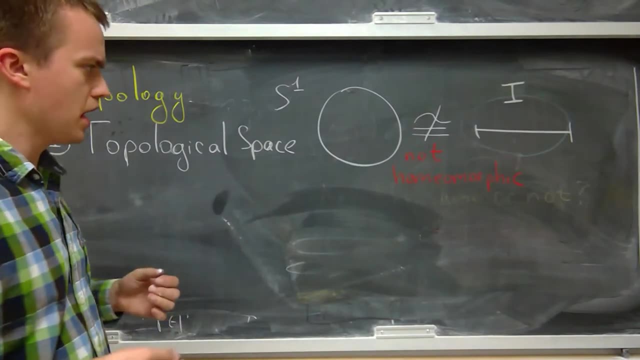 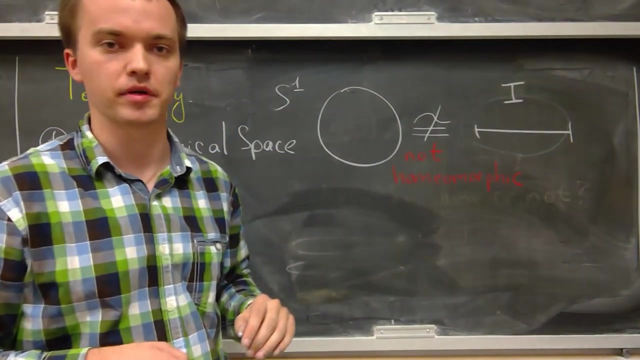 space. so topological space we just introduce like an abstract mathematical space and for this space we're going to have, we want, uh like, on this space we want to define such mappings. but if you want to define mappings with certain properties, we want to discuss after topological. 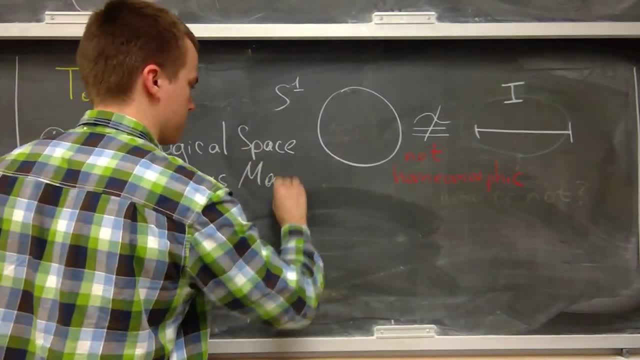 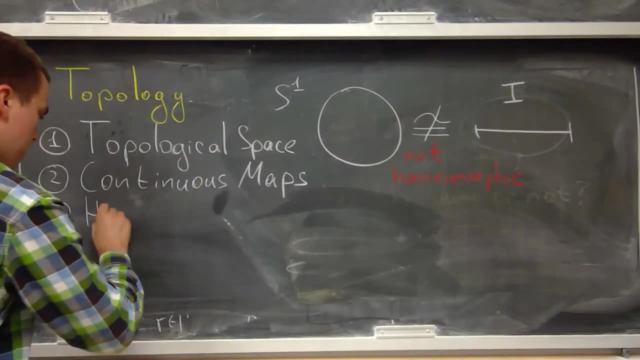 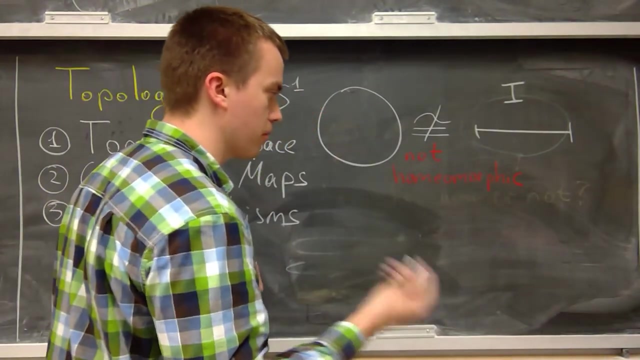 space with this continuous map. after we're going to discuss continuous maps, uh, the next thing we want to discuss: homeomorphism. and when we have our homeomorphism, so we're saying that these two spaces is not homomorphic. so in terms of topology, it means, if i will have 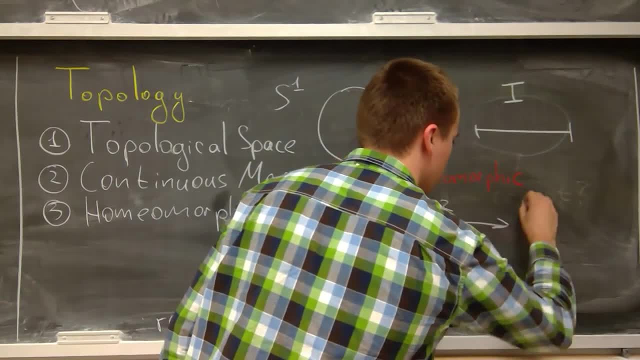 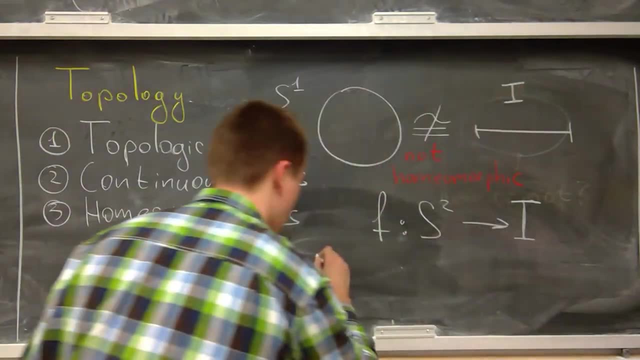 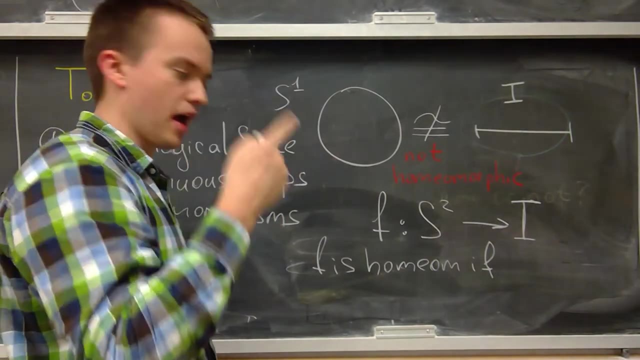 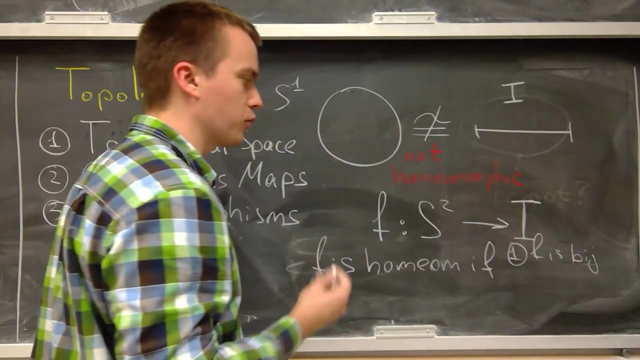 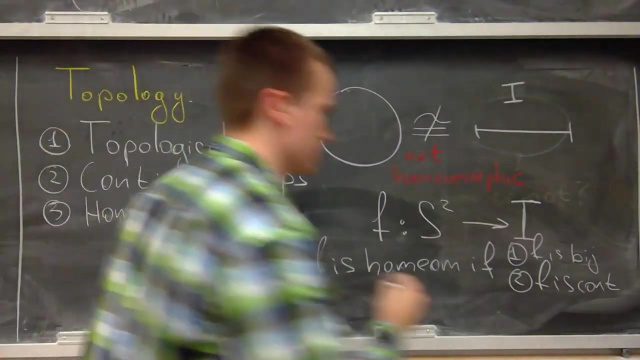 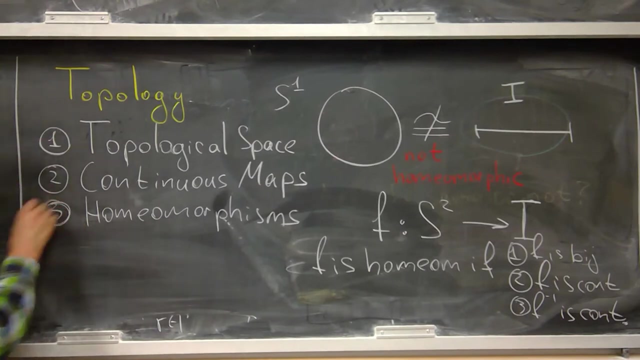 map f between s2 to interval, then i'm saying that f is homeomorphism. if i have two properties: first, f is bijective, second one f is continuous and the third one, inverse of f, is continuous. so by introducing this three concept on the- i will say- third video, you will be able to understand. 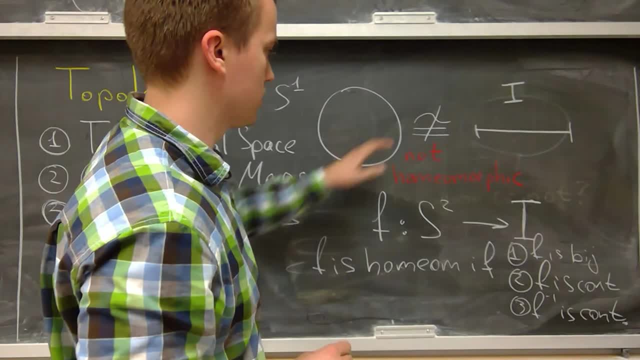 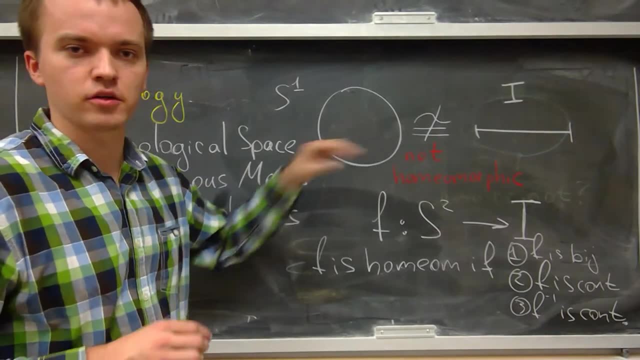 what is, what does it mean to be homeomorphic? and let's show me the last thing. let me show that these spaces are not hammer homeomorphic, um. so, first of all, we want to understand what is, what does it mean to be homeomorphic? let's say the fourth thing that you want to study. we want to study connectedness. 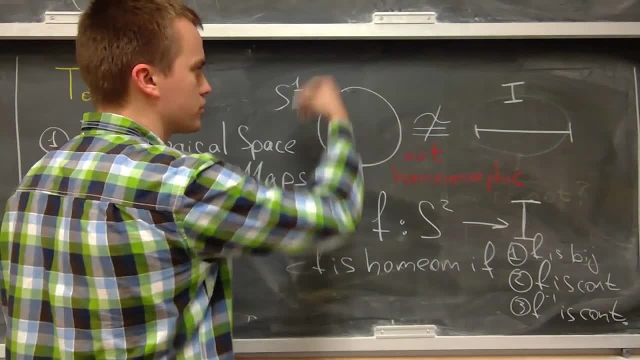 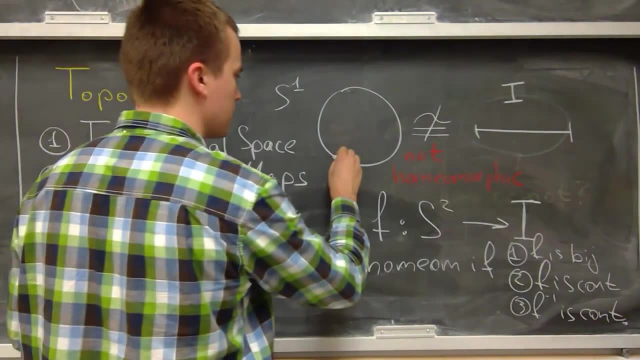 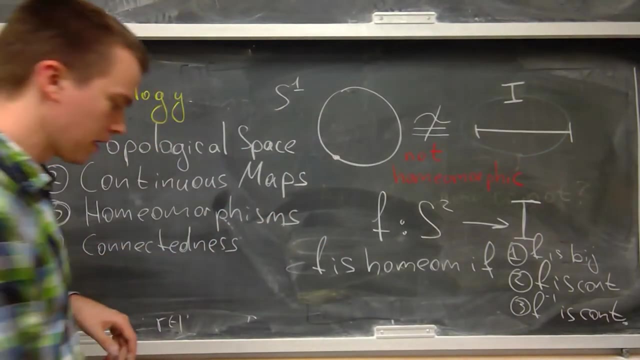 and for connectness means that, for example, circle and unit interval is one connected. they have only one connecting component. why? because you can see, you cannot kind of separate your space into two disconnected component- and again we're going to give definitions later. and the cool property about 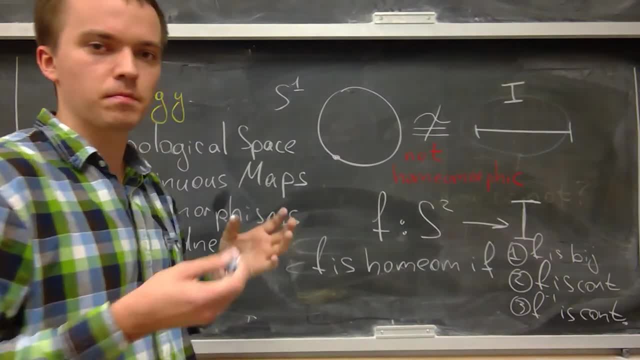 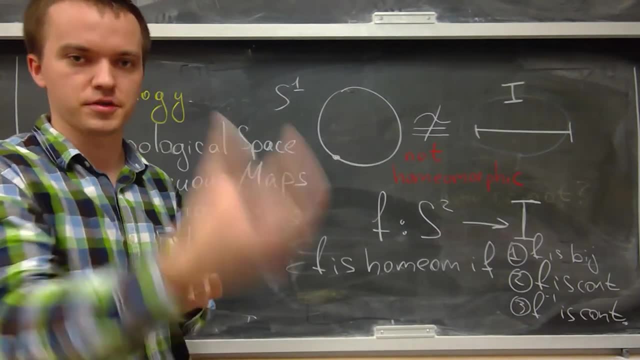 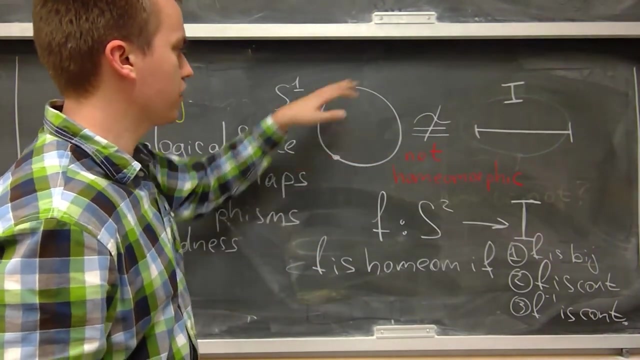 homeomorph, uh, homeomorphism that some topological, like structure, some topological feature of our space are going to be saved under homeomorphism. so if uh this like two spaces homeomorphic, it means like, uh, if they're like connected, then you can see that. 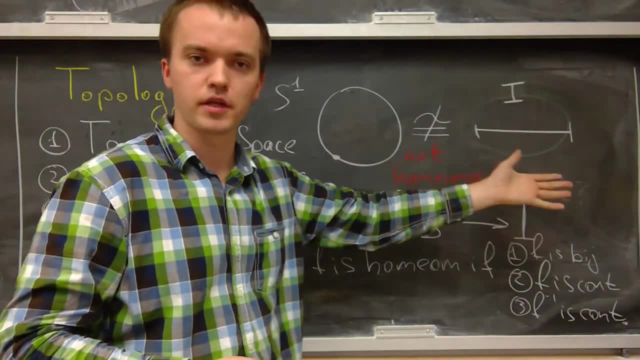 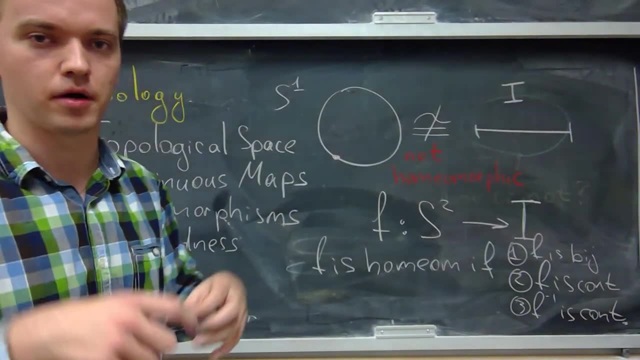 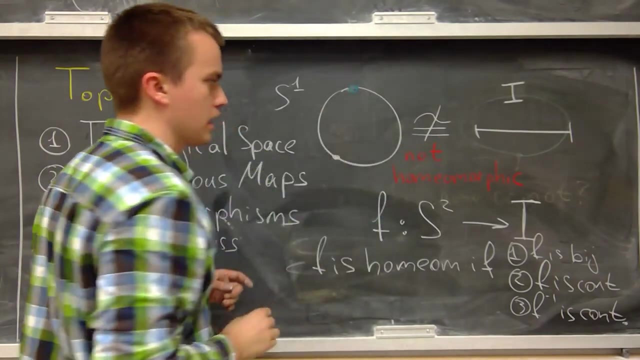 when you map one space to another one, the another space must be connected. if one space is bounded like a compact, another space also must be compact. so complicated means like closed and bounded. but here you can see if i'm going to remove here one point. since f is bijective, i'm going to remove. 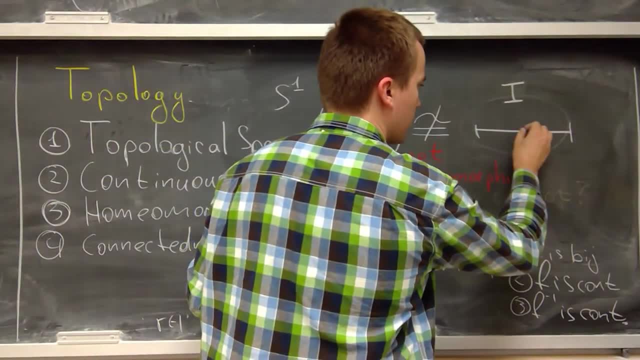 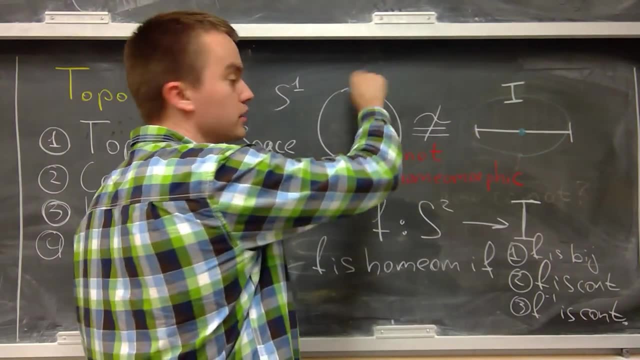 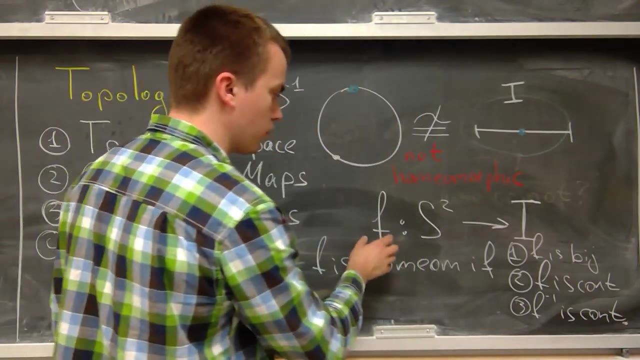 only one point on my unit interval and let's say, uh, that i'm not removing like boundary point, and i can do this, because if i remove boundary points i need to just remove another point, and then you can see that if there were homeomorphism between s2 and i, or in other words,